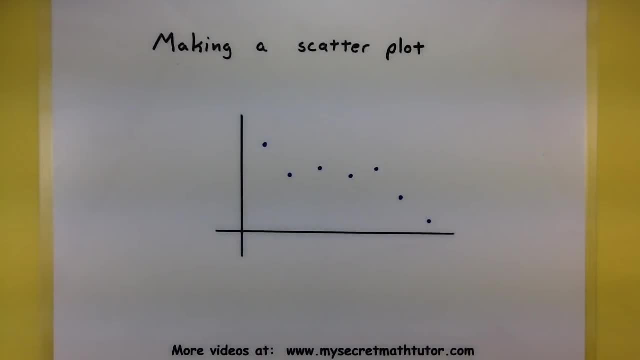 Hello and welcome to My Secret Math Tutor. In this video I want to show you how to make a scatter plot. So these are really great types of plots that we can use to help see relationships in our data. To be a little bit more specific, in a scatter plot we use 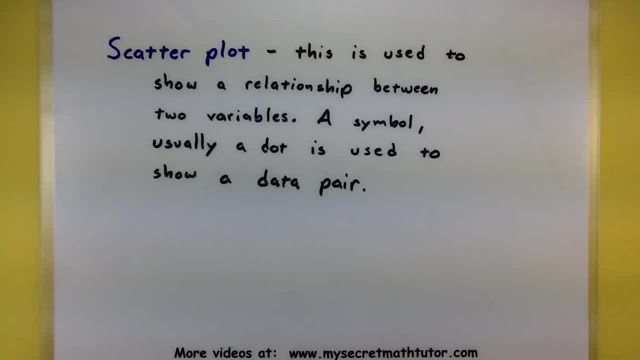 these to show a relationship between two variables. Now, usually a symbol, usually a dot, is used to show an individual pair of data. Let's look at some other terms that are also used when describing these scatter plots. We'll take the data and take both of our variables. 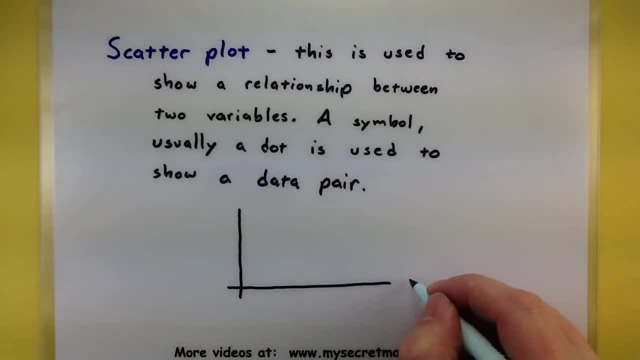 and represent them along both of these axes. here, On the bottom one, we call this our x-axis. This is where we'll display our independent variable. Along the other line are y-axes. We'll display the second variable. We'll call this our dependent variable. Now you 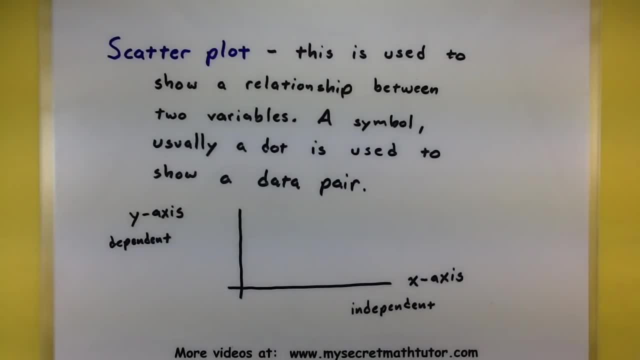 might be curious. how on earth do we know which one is the dependent variable? How do we know which one is the independent variable? Well, think of it this way: The dependent variable will change as a result of what the independent variable is doing And when we 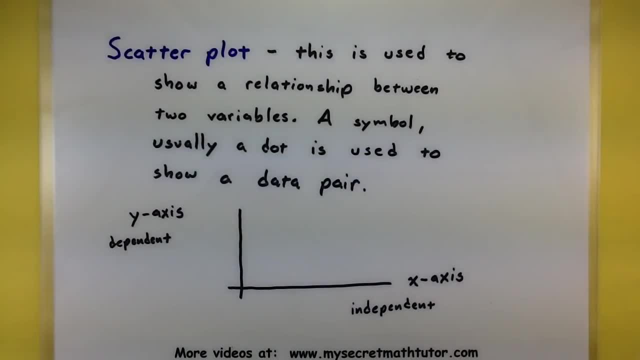 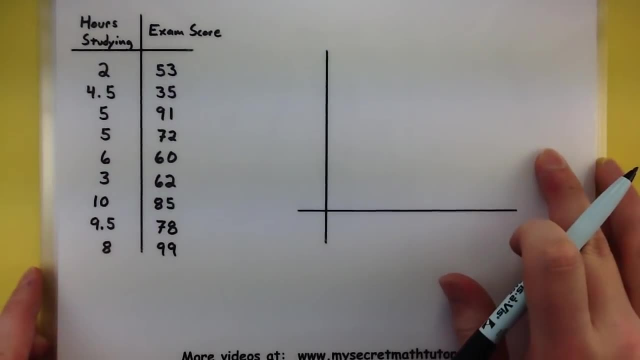 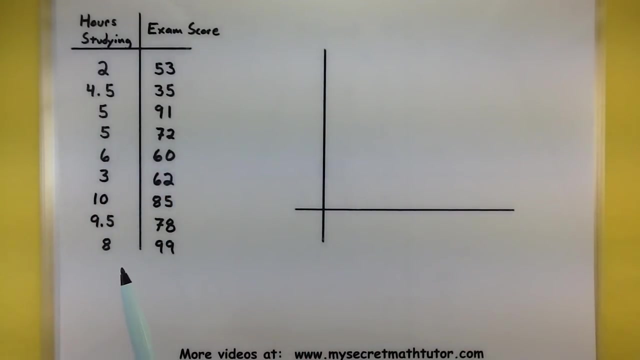 get to my example, you'll probably be able to more clearly see which one is depending on the other one's value. All right, let's give it a try. So we want to create a scatter plot for the following data, And this chart or table here just represents the hours of studying and a particular exam. 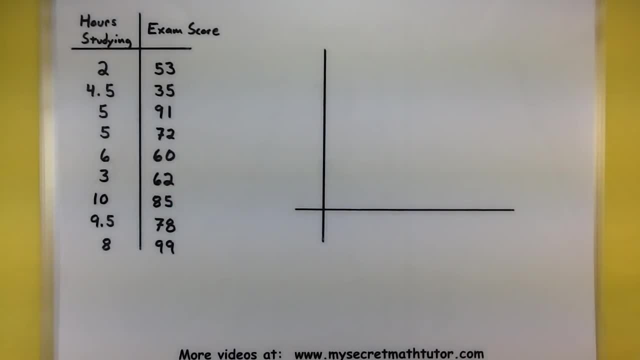 score that some students had. So which one of these would depend on the other one? Well, we would think that whatever exam score they got probably depended on the hours of studying. So we will say that the hours of of study are independent and the exam scores are dependent. 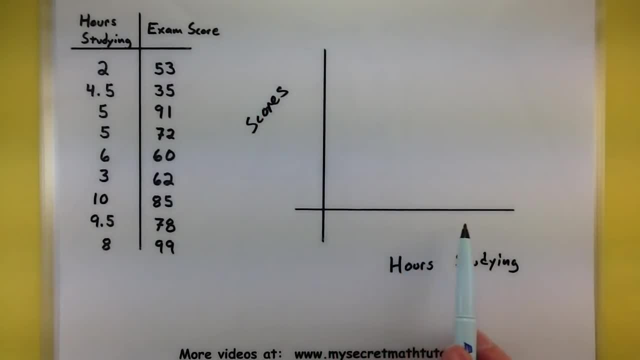 There we go Now. it's also important to mark out a scale so we can put all of these data values in here. And looking at the hours of study, it looks like somewhere between 0 and 10 hours is probably good. So let's mark off 10 little tick marks. 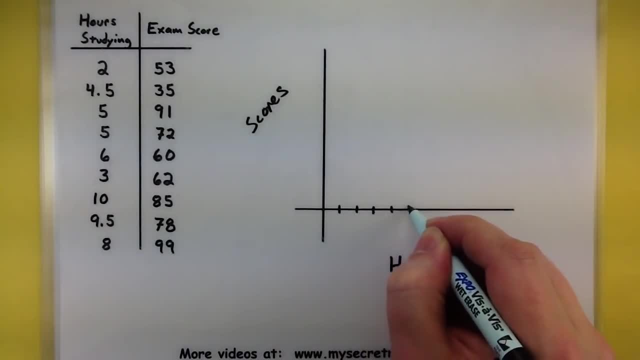 So 0,, 1,, 2,, 3,, 4,, 5,, 6,, 7,, 8,, 9,, 10.. 1,, 2,, 3,, 4,, 5,, 6,, 7,, 8,, 9, oops, got an extra one, 10.. 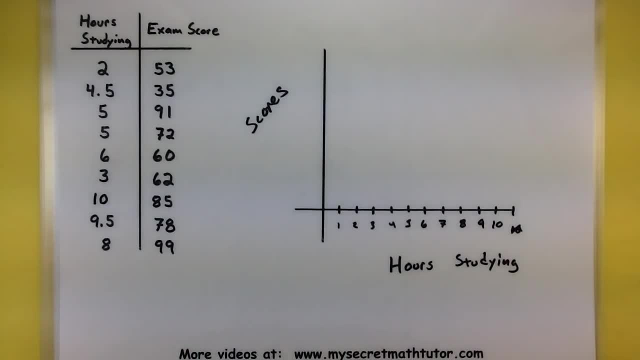 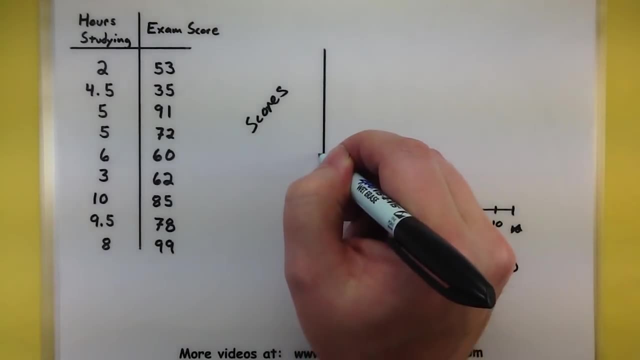 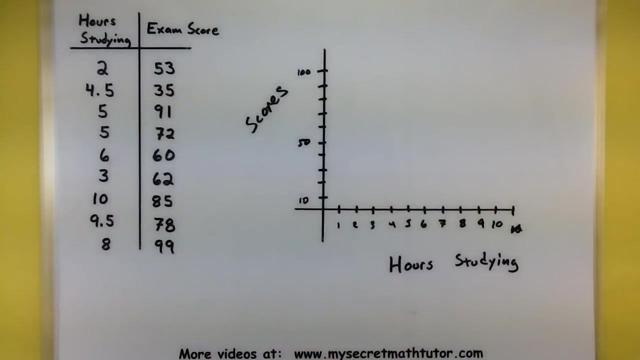 All right Along the other side. This is where our exam scores will go. Let's just do 0 to 100.. So 10, 20,, 30, 40, 50,, 60, 70,, 80, 90, 100. 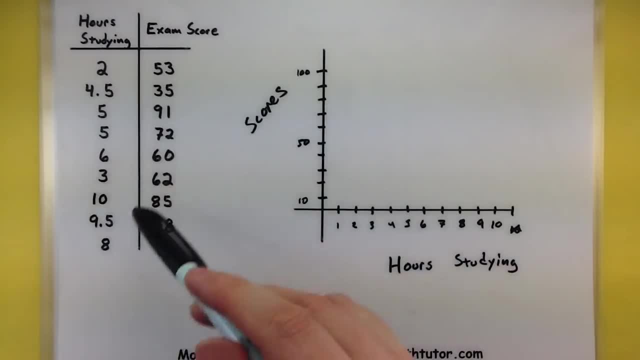 OK, looks good. Now. the way this works is: we want to put a data point at the intersection of hours and scores, so that that one point represents a pair of data. Let's start off with the first one. So we want to put two hours of studying and a score of 53. 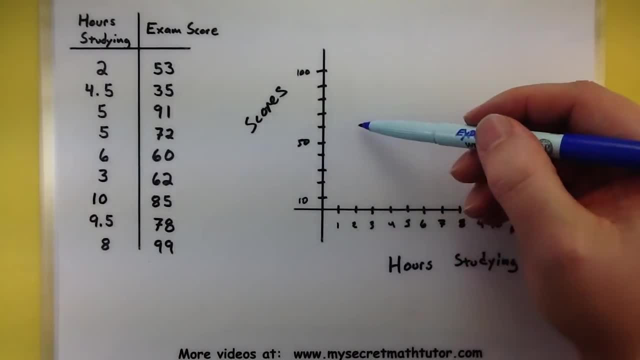 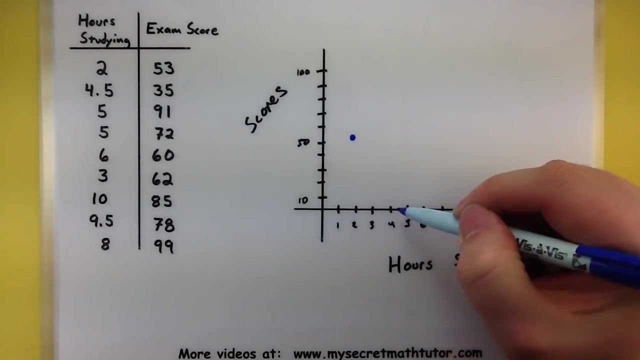 So we'll first find the hours of studying. There's our 2. And we'll put a dot where it intersects 53, so just a little bit above the value of 53.. Not bad, Let's do this again. So we've got 4 and 1 half 435, so 4 and 1 half halfway between. 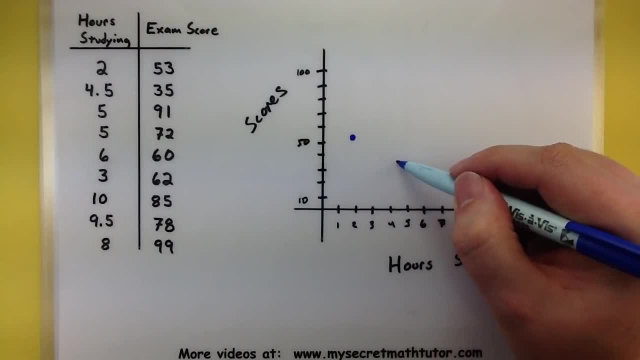 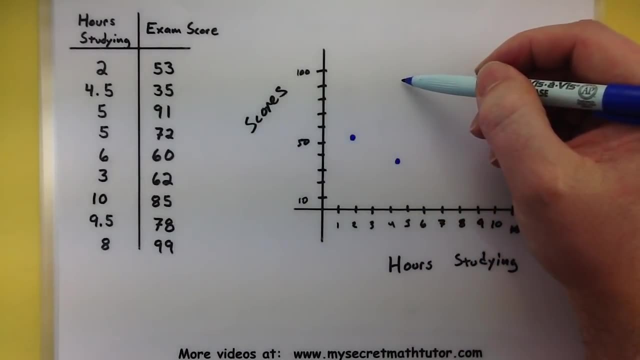 Up to 10,, 20,, 30, and a half- Not bad OK. Up to 5.. 5 needs to go all the way up to 91,, so way up here, Let's keep going. We also have 5, which is at 72.. 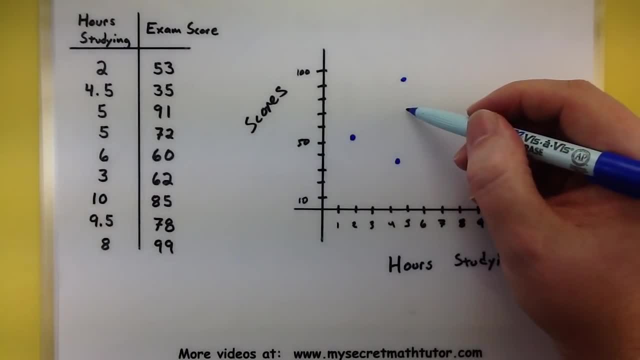 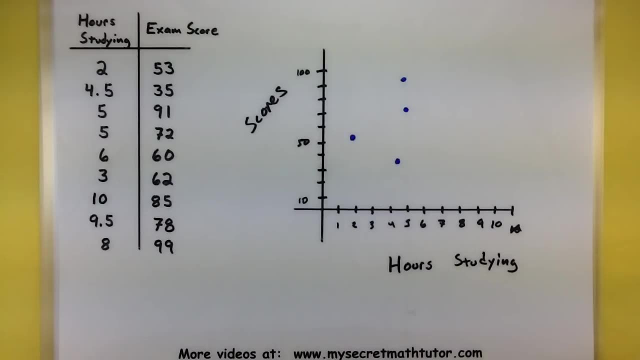 Let's see so 50,, 60,, 72.. Notice how we get two values of both for 5, and that's OK. Sometimes that can happen with these scatters. Let's see 6,. we need a dot at 60.. 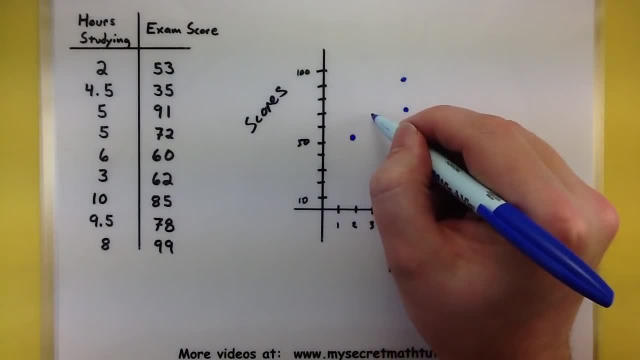 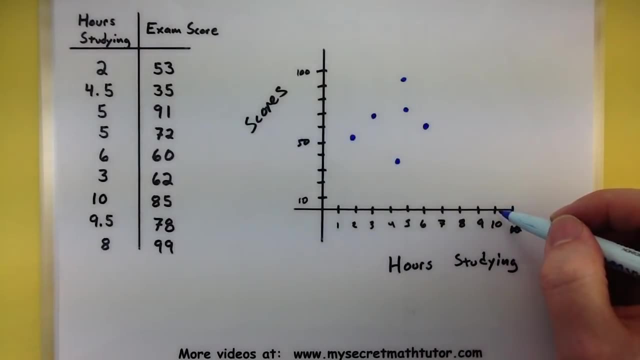 3,. we need one at 62. Let's see 10, over here. we need one at 85. There's 50,, 60,, 70,, 80,, halfway 85. Let's see 9 and 1 half, so halfway between these two.